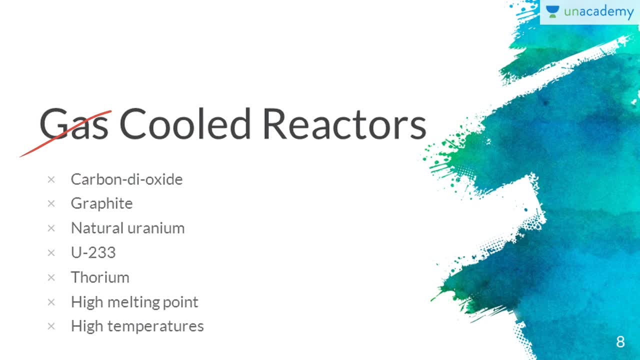 So gas cooled reactors, let's start with the gas cooled reactors. Gas cooled reactors which were founded were with the presence of carbon dioxide gas as coolant, with the pressure of around 16 bar, and graphite as a moderator. It was developed in Britain during 1956 to 1969.. 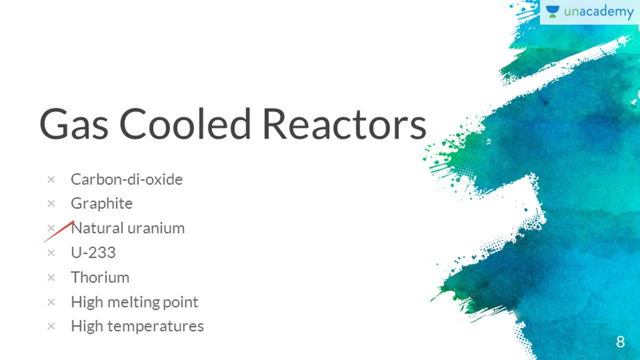 The fuel was a naturally uranium which was clad with a lot of magnesium, called the bag box. The graphite water rated helium cooled is designed. Helium cooled reactor is designed to use the U-233 as a fissile metal reactor material and thorium as the fertile material. Initially, the system would have to be filled. 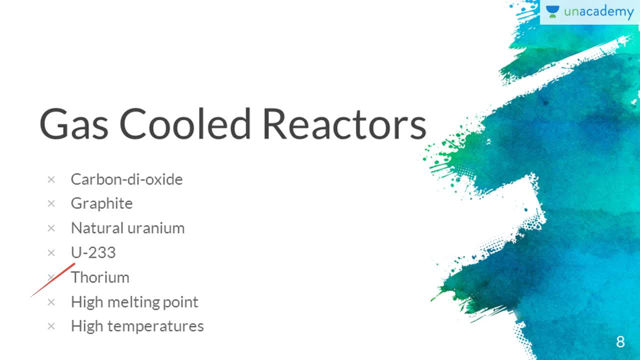 with U-235 until sufficient U-233 is available for make-up fuel. Because of very high melting point of graphite, these fuel elements can operate at very high temperature and it is possible to generate steam at conditions equivalent to those in modern coal fire power plants. 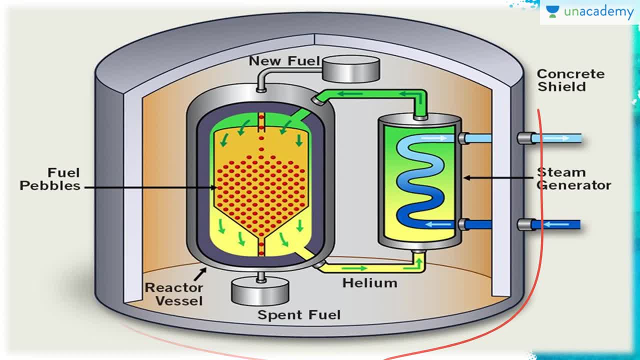 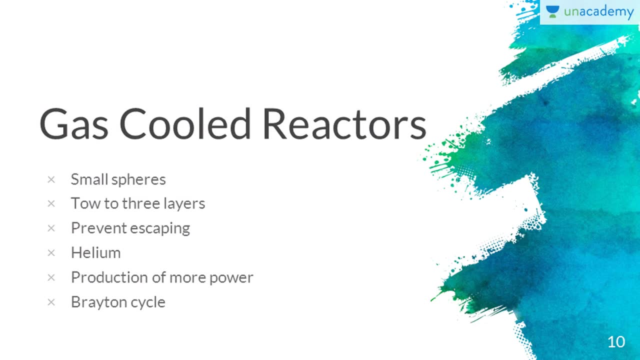 So this is how the gas cooled reactors are available and how they are there. This is an image representation or image depiction of a gassed cooled reactors, So let's start with it again. So the basic fuel forms? they are the small spheres of fissile and fertile. 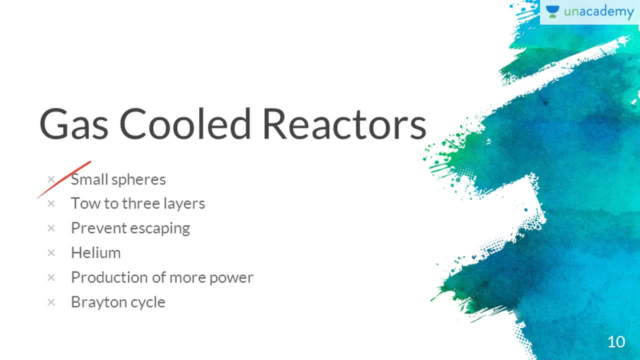 metal as carbides. The fissile spheres are of 0.35 to 0.5 mm in diameter and fertile spheres are 0.6 to 0.7 mm in diameter. So these are the gas cooled reactors. So this: 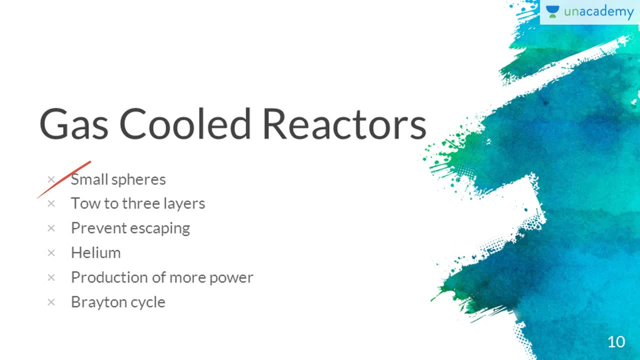 is the gas cooled reactor. Each sphere is coated with 2 to 3 layers of carbon and silicon carbide to prevent fission products from escaping from the particles. Helium is a suitable coolant in that sense as it is chemically inert and has good heat transfer characteristics, and 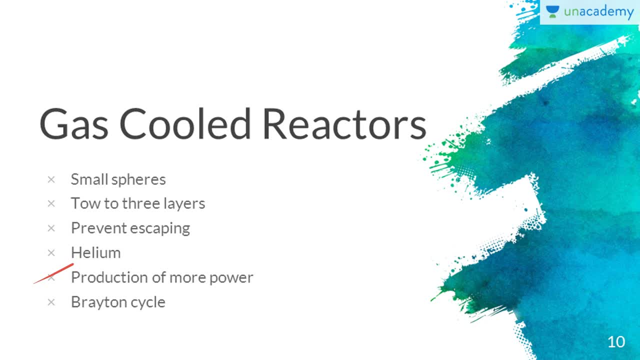 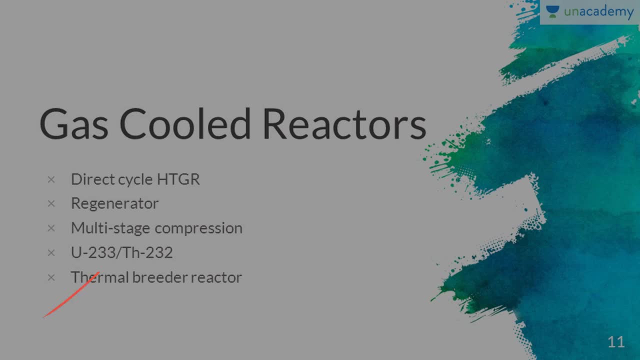 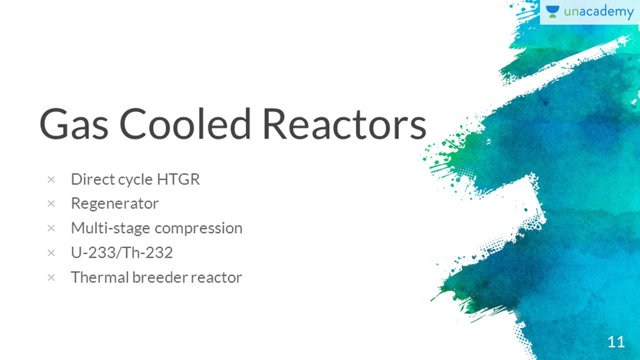 low neutron absorption. Being a monatomic gas, it can produce more power for given temperatures in the Brayton cycle, as well as for higher efficiency. So let's move on to the direct cycle. HTGR, that is nothing but the helium cooled graphite moderated reactor, So it is a gas turbine power plant which incorporates a regenerator. 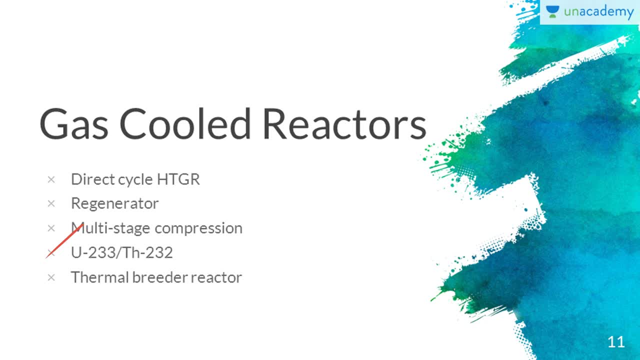 and a multi-stage compression with intercooling. These cycles, or these turbines, consist of cycles such as pressure ratio, turbine inlet pressure, which is around 50 bar, turbine inlet temperature, which is around 900 degree centigrade, and the compressor inlet temperature, which is 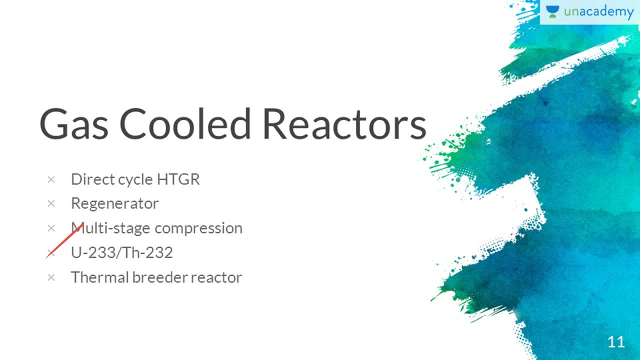 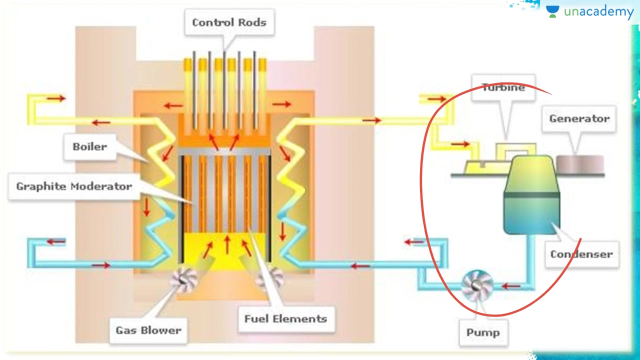 around 50 degree centigrade. the temperatures at other points are shown in the like computer numerical column. and all so with u233 and thorium 232 spl, the gas cooled reactors. they function as a thermal breeder reactor. so this is what the glass current reactor is. you can see here the 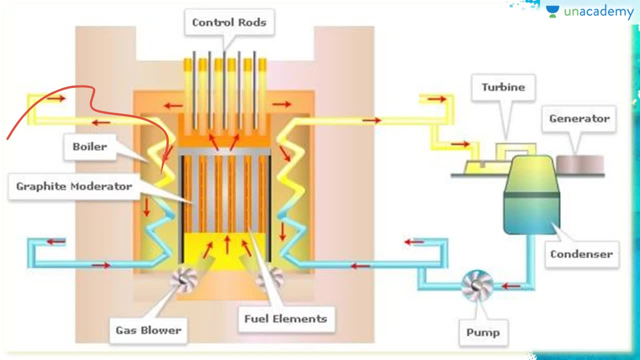 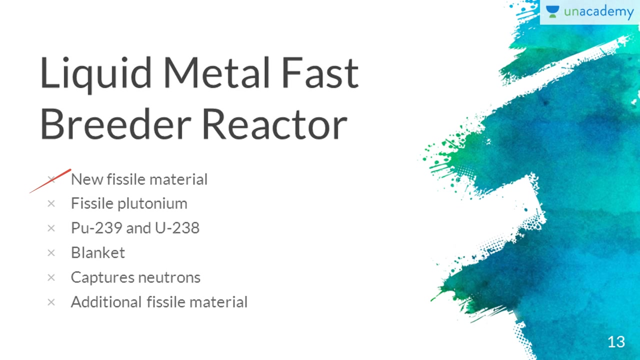 turbine generator condenser. so this is how it actually. it acts as a boiler. also see here you can see the gas blower and the fuel elements passing over here to the control rods. so let's move on to the liquid metal fast breeder reactor. so this fast breeder reactors are designed to. 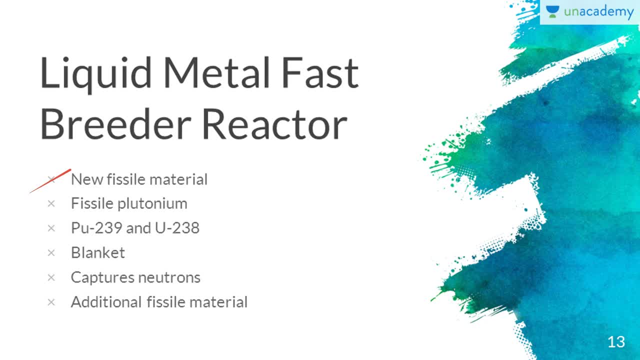 create or breed new fissile materials while producing useful electric power more, most of them produce fissile plutonium for fertile uranium 238. the fuel rods in the core region thus contain a mixture of fissile plutonium 239 and uranium 238. the active core region is surrounded by a blanket of fertile uranium 238. this blanket region captures 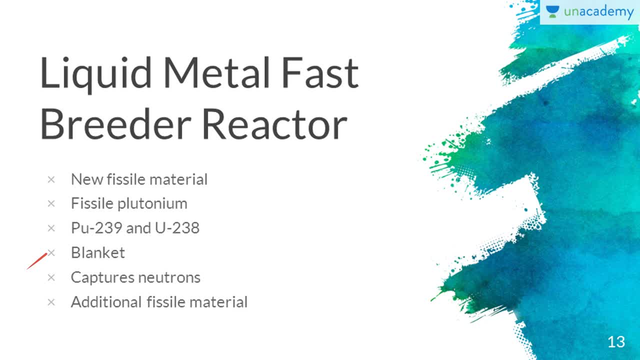 neutrons that would otherwise be lost through the leakage, thus producing additional fissile material. so the doubling time is the time required to produce the fissionable nuclei twice the number of the fissionable nuclei consumed. the high concentration of fissile fuel and the absence of moderator makes the core of a fast reactor smaller than a thermal. 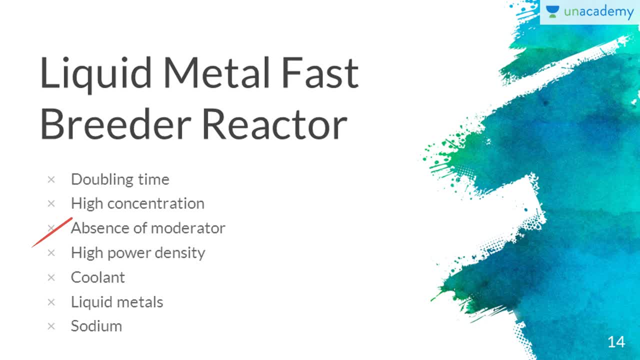 reactor of the same power with a high power density. thin fuel pits are used to minimize the temperature drop through the fuel. a coolant with excellent heat transfer properties is required to minimize the temperature drop from the fuel surface to the coolant, and also it must be non-modernity. this rules out water, and the best coolants for fast reactors are liquid metals such 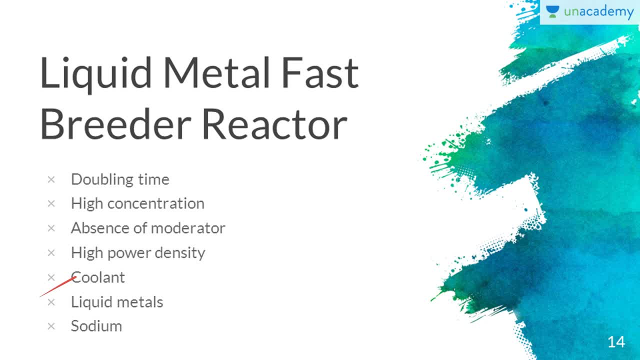 as liquid sodium. liquid metals have the additional advantage that their boiling points at atmospheric pressure are very high, so that most of them can be used that used as unpressurized in the reactor. sodium is the most common used coolant for fast reactors. so you can see the 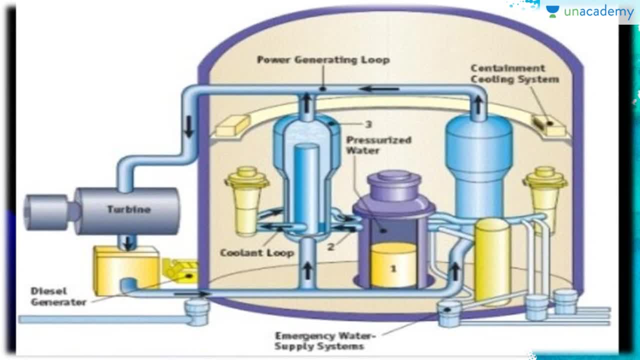 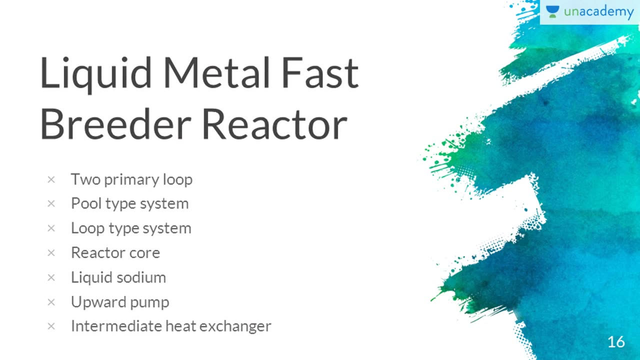 liquid metal fast breeded reactor or the liquid metal fast 무� jego, too high current reactor. so it consists of a two primary loop: the breeder reactor, namely one, namely the pool type system, and the other, namely the loop type system. in the pool type system, the reactor core, the primary pumps, are the immediate intermediate heat exchangers. they are quarried artificially, so that means they are conditioning pressure and the water will also Pablo. 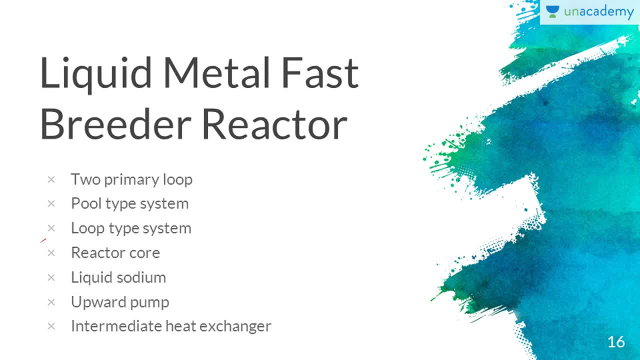 it will equilibrate the地域. liquid metal fast breeder base, such as the liquid metal scorpion which was used by Barry, all placed in a large pool of liquid liquid sodium contained in the reactor vessel or the reactor coil. the liquid sodium is discharged from the intermediate heat exchanger to the pool. it is 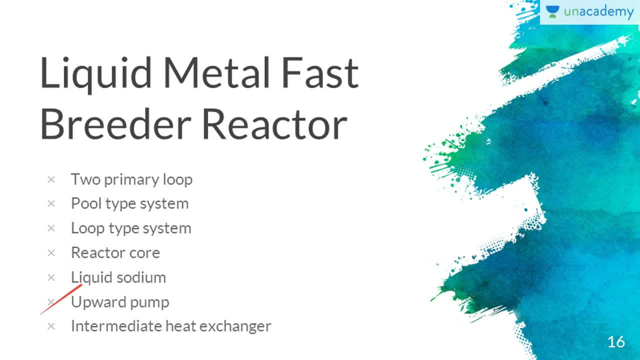 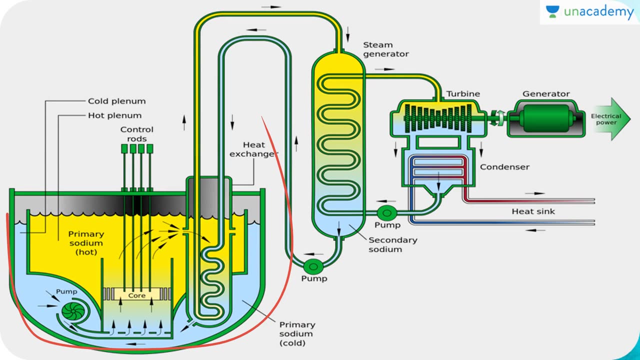 then pumped upwards to the core and it re-enters the heat exchanger in the loop system. the intermediate heat exchanger is located outside the reactor vessel, so this is how the breeder reactor will be there. you can see the control rods, which is there are two types of control. 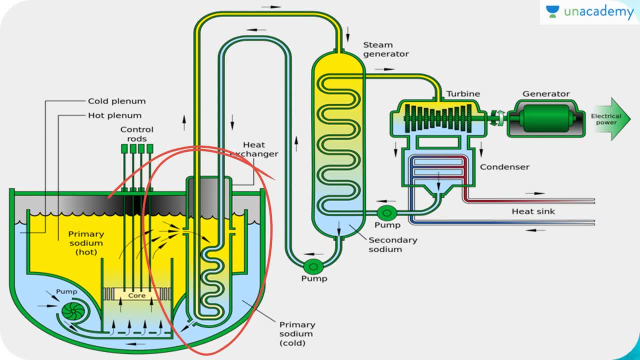 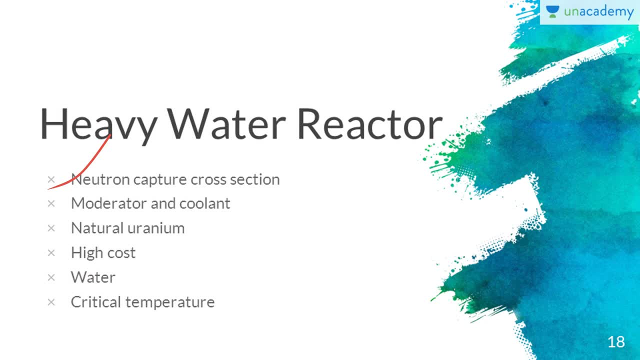 rods, namely one is placed outside the reactor and another is placed inside the reactor. so let's move on to heavy water reactors. they are very low neutron capture. cross section of heavy water makes it an excellent moderator and coolant and permits the use of natural uranium up to 0.7 percent of q to 35. as fuel reactors of this type have good neutron capture and 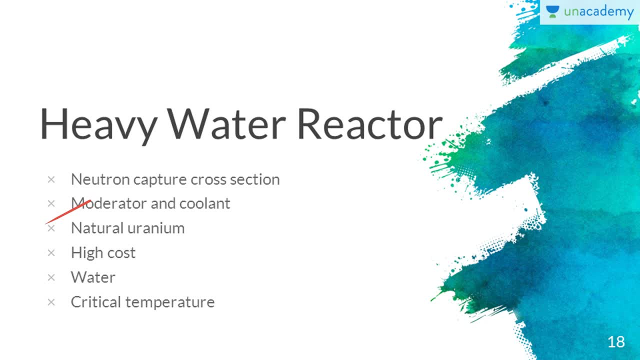 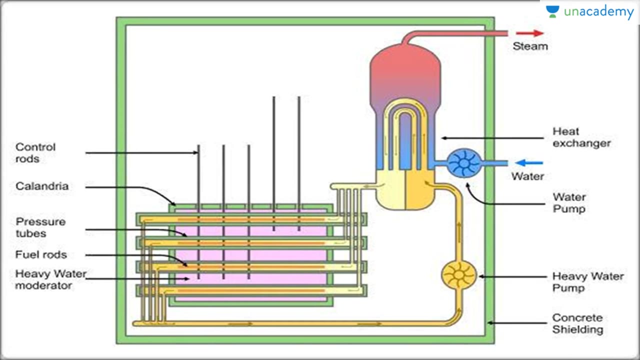 economy and they result in good reading ratios as well as high fuel burn up and a reduction in fuel cost. the disadvantages of heavy water are it's very high cost and, like water, it's critical temperature limitation. so you can see the image representation of a heavy water reactor over here. 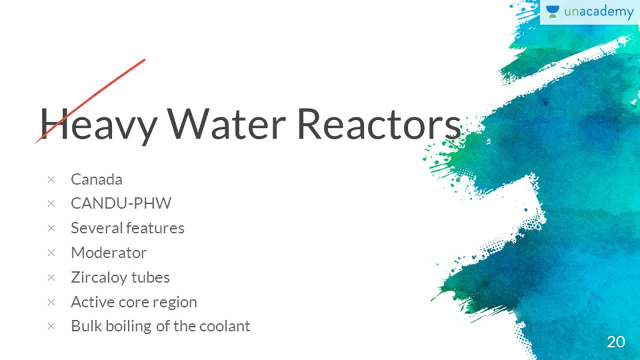 so heavy water reactors. heavy water moderated and cooled reactors have been extensively developed in canada and they form the basis of the nuclear power program in that country. they are called candu hyphen, phw, which means canadian deuterium uranium pressurized heavy water reactors. 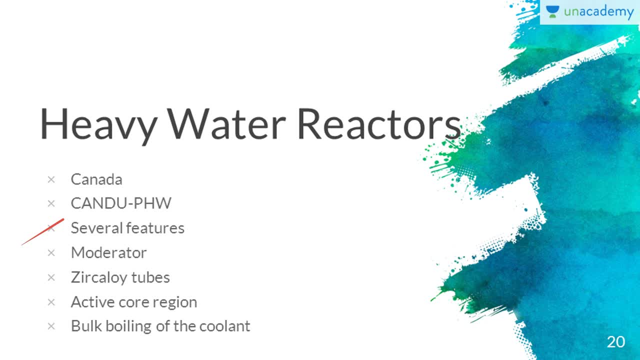 these reactors, they have several features that distinguish them from the other types. the moderator is contained in the cylindrical steel vessel called the calendria, with a large number of zirculoid tubes through it, parallel to its axis, which is very horizontal, the active core region is approximately six meter high, with a diameter of seven to eight meter. 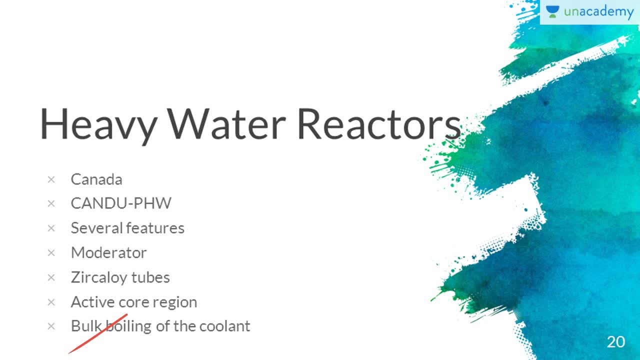 the d2o coolant enters the regular array of pressure tubes at 260 degree centigrade and 110 bar and it flows through the fuel elements, which leaves the pressure tubes at 320 degree centigrade and the net efficiency will be about 29 percent, like the pressure water pressurized water reactor. 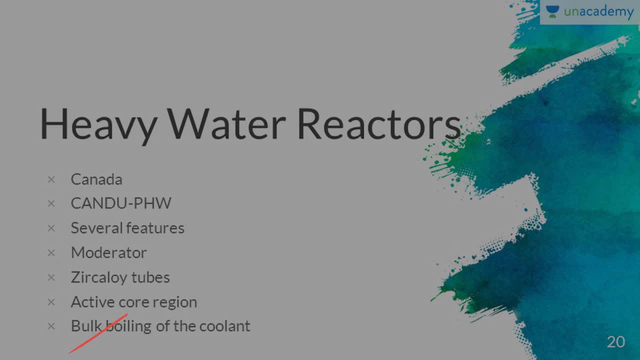 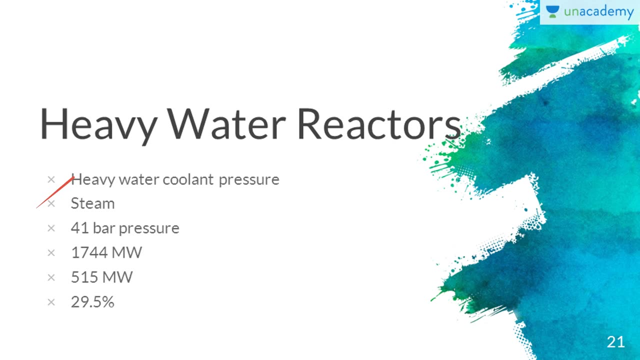 there is no bulk boiling of coolant in heavy water reactors. so the heavy water reactors, they have a heavy water coolant pressure in the reactor which is about 88.3 bar and the inlet and the outlet temperatures are around 250 degree centigrade to 280 degree centigrade respectively. in the heat exchanges the steam is generated at 41 bar pressure. 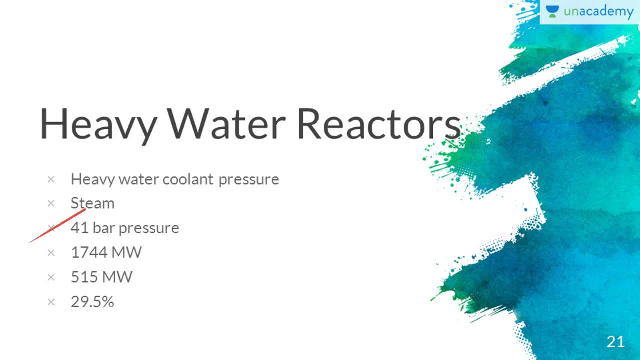 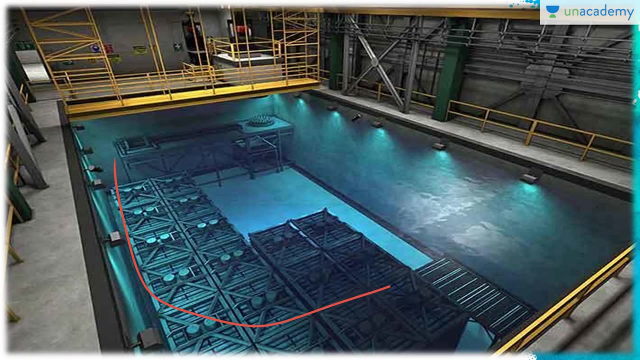 251 degree centigrade. the thermal power of each reactor is 1744 megawatt and the electrical output is 550 megawatt, which gives a thermal efficiency of around 29.5. so you can see the housing of a heavy water reactor over here. you can see the housing. 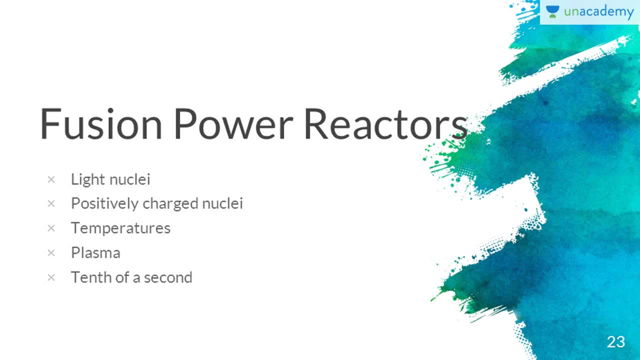 which is present here. so let's move on to our last reactor, namely the fusion power reactors. the fusion of light declaring to form a heavy nuclide releases energy to cause fusion. ITI is necessary to accelerate the positive charge topiel to high kinetic energy in order to overcome 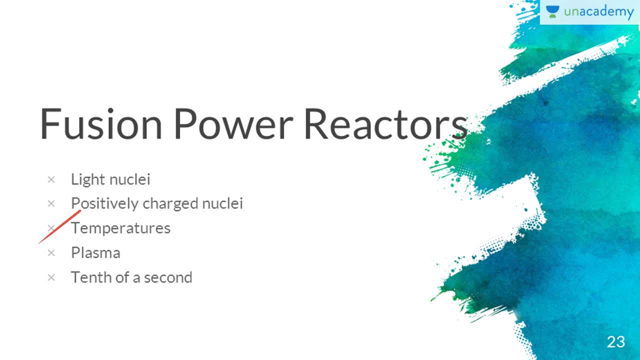 electrop constellations by raising the temperature and coldernap just one half of the Щn to hundreds of millions of degrees, resulting in a plasma plasma. the plasma must be prevented from contacting the walls of the container and must be confined for about tenth of a second, having a density of around 10 power 15. 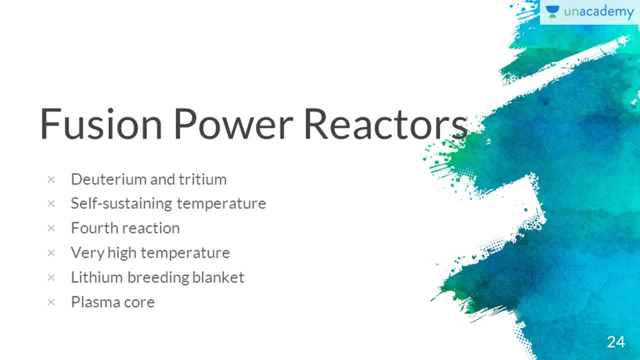 ions per centimeter square. so the fusion power reactors. they are dependent on the deuterium and the tritium, or the tritium deuterium, being a very stable, heavy isotope of hydrogen, is present in natural water. is the main fuel for a. 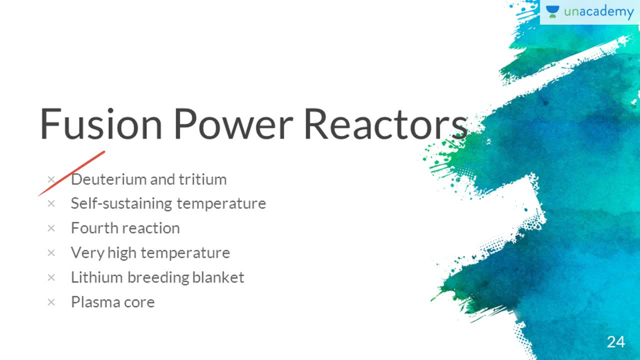 fusion reactor. it has self-sustaining temperature, which is a temperature of around 15 to 10 plus 6 Kelvin, which releases around 17.6 mega electron volt per reactions. the first two d2d reactions occur at 500 to 10 plus 6. 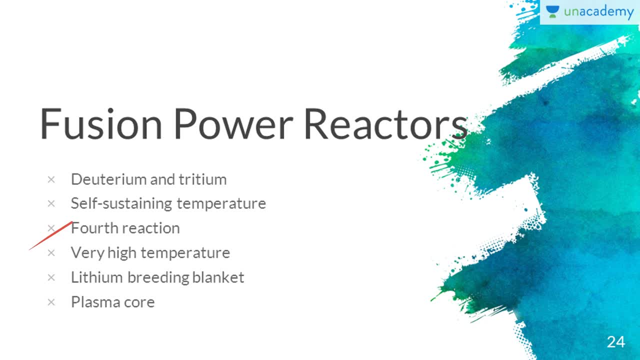 Kelvin and release energy which is around 3.2 to 4.0 mega electron volt. and the fourth reaction releases very high energy, 18.3 mega electron volt. but it requires a very high temperature, that is thousand to 10 power, 6 Kelvin for fusion the tritium it does. 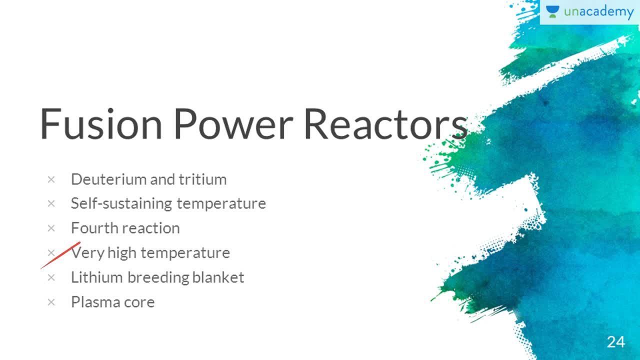 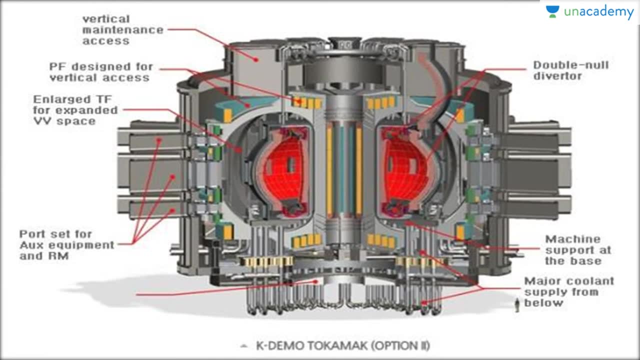 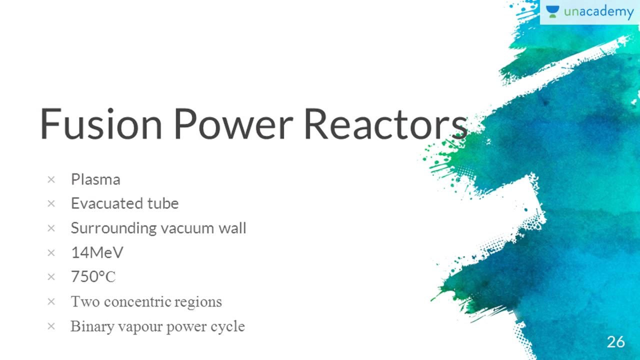 not occur abundantly in nature. however, it can be produced for a lithium breeding bracket that surrounds the plasma of the fusion reactor. so you can see the fusion reactor over here. you can see this is the plasma which I was talking about in the last slide, so the fusion power. 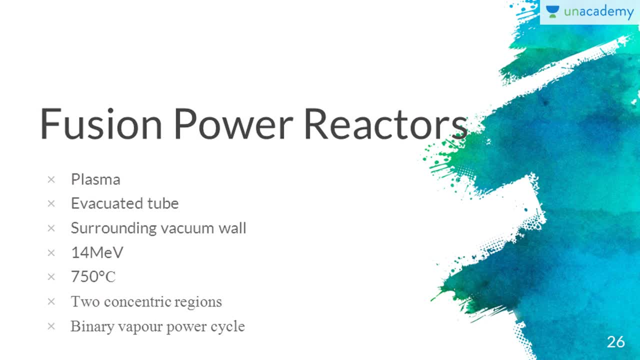 reactor is aocal tube and this is the fusion. knew that the nuclear reactors actually have this plasma contained inside a evacuated tube of about four meter. the sorority vacuum wall is through which it is. there is a round 4 beat electron bolts neutral for the plasma pass is maintained- about 750. 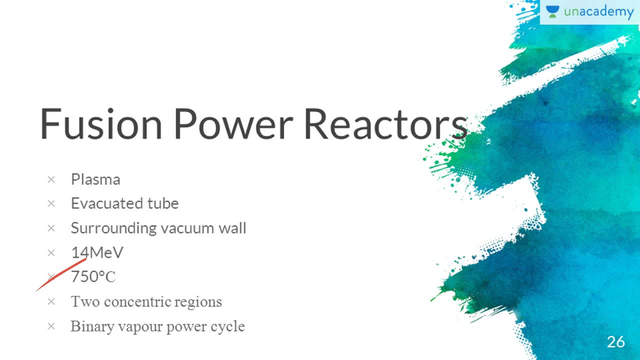 degree centigrade and outside this wall are 2 concentric regions. the lithium breeding border at the magnetic shield. the tritium is manufactured to the lithium bracket. our large cryogenic superconducting backaye's off around 17.1 cucumbers. do TRI anticipate interruption over a falcon or effervescent magnetism. Siberian fusionhuhl appears in the same. 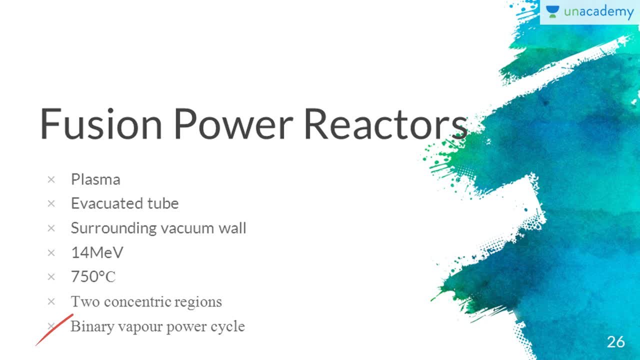 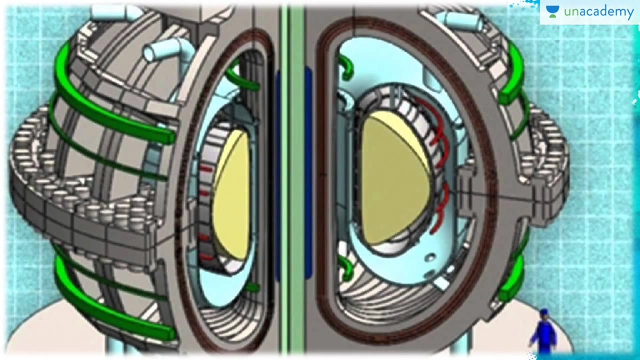 to 8 meter diameter, maintain the magnetic shield, the binary vapor power cycle. they consist of a potassium topping cycle as well as a conventional steam cycle. it includes a tritium recovery system. so the advantages. so this is an overview of the animation drawing of a fusion power reactor. 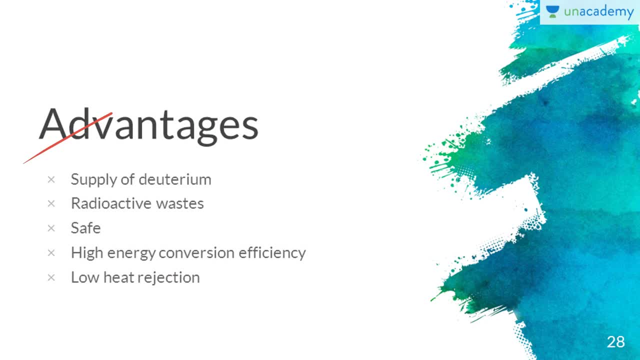 so the advantages of the fusion power plant are: it helps with the supply of deuterium when it is almost inexhaustible. the radioactive wastes are not produced in this fusion power reactor. it is very safe to operate. it has a high energy conversion efficiency of around nearly 60.